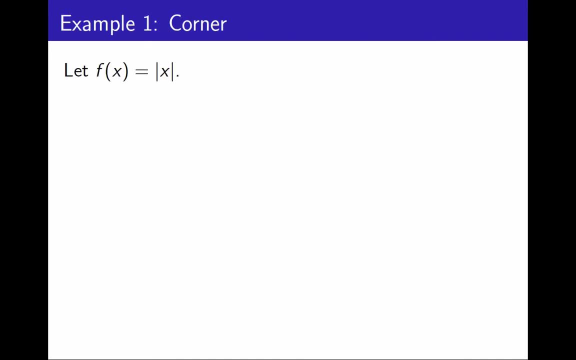 For my first example, consider the function: f, defined by f, equals absolute value of x. I want to know whether f is differentiable at 0.. Let's try to compute the derivative at 0, as the limit, as x approaches 0, of f minus f over x minus 0.. 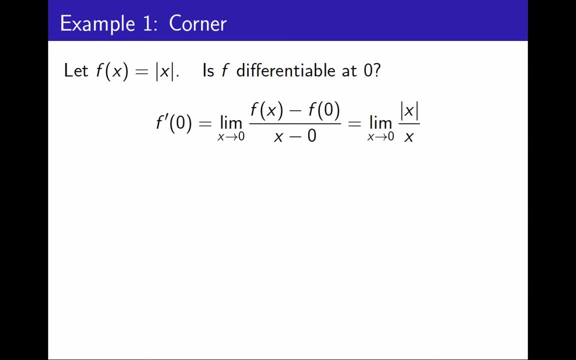 Using the definition of f. this is the limit of absolute value of x over x. Since we have the absolute value of x, it is easiest to break it into two cases: When x is positive, as x is approaching 0 on the right. 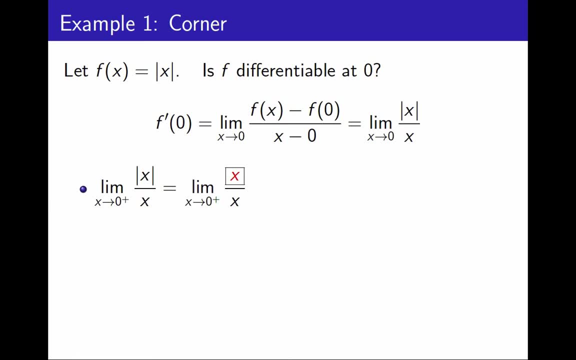 the absolute value of x is simply x and the limit is 1.. On the other hand, when x is negative, as x is approaching 0 on the left, the absolute value of x is minus x and the limit is minus 1.. 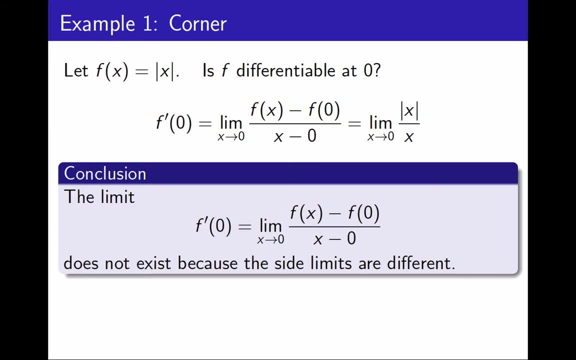 In conclusion, the derivative at 0 does not exist because the two side limits in the limit definition of derivative are different. Remember that derivative represents slope. I can interpret this by saying that at 0, there is a slope on the right and a different slope on the left, so to speak. 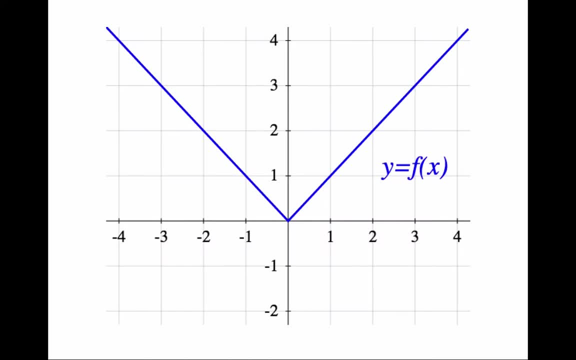 And yes, that is what the graph looks like. The slope at 0 seems to be 1 if I look at 0 from the right and minus 1 if I look at 0 from the left. The graph has a sharp edge, a corner. 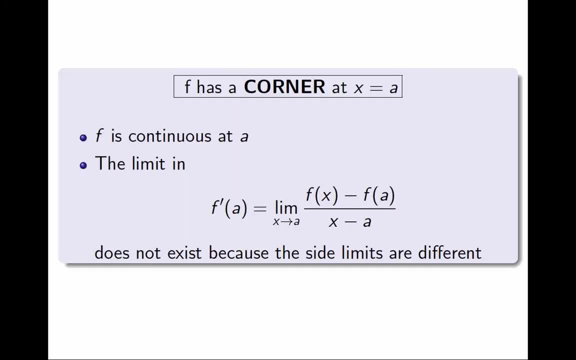 And in general a function f will have a corner at x equals a when f is continuous at a, but the limit in the definition of derivative f' does not exist because the side limits are different. For the second example I will look at the function g. 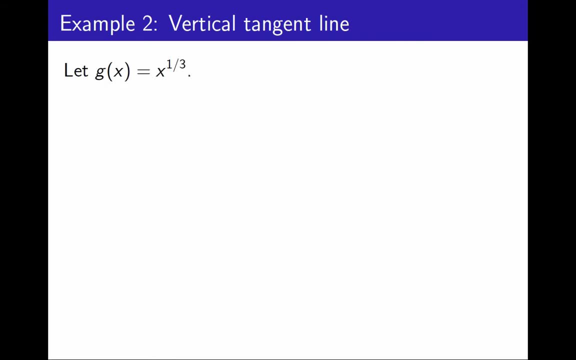 defined as g equals x to the 1 third. I want to know whether g is differentiable at 0.. Again, I try to compute the derivative g' from its definition as a limit, Using the expression I have for g. this is the limit as x approaches 0, of x to the 1 third over x. 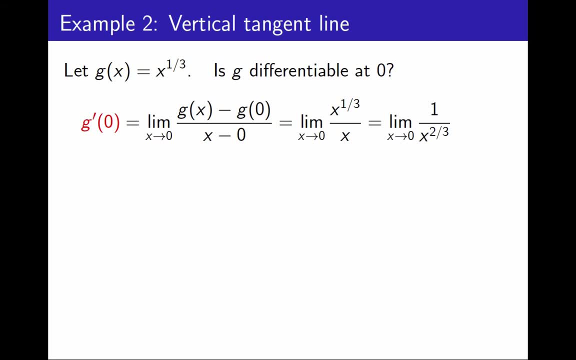 which is the limit of 1 over x to the 2 thirds. This limit is infinity because the denominator has limit 0 and is always positive. Now remember that derivative means slope. What does infinite slope mean? A line with infinite slope is a vertical line. 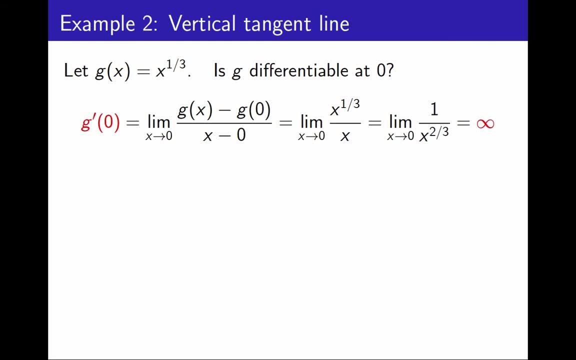 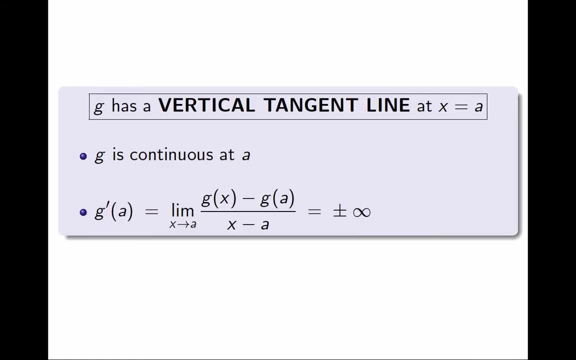 so this suggests the graph has a vertical tangent line, And indeed this is what the graph looks like. More generally, I will say that a function has a vertical tangent line at a point a, when the function is continuous at a and the derivative at a, computed from its definition as a limit. 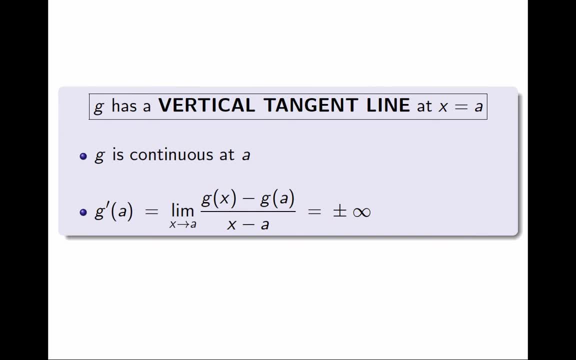 is plus or minus infinity. In the example it was plus infinity, but minus infinity would also produce a vertical tangent line. We are not done yet. There is a little bit more to add to the concept of vertical tangent line. Let's go back to the example. 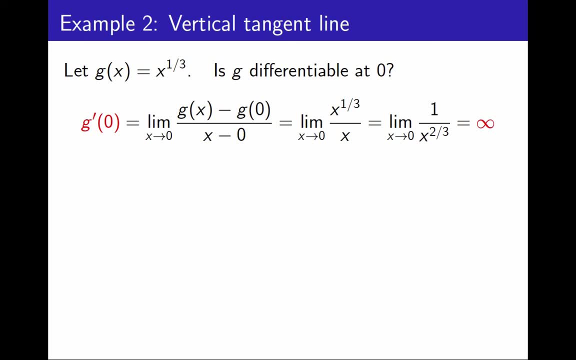 I can look at it in a different way. Whenever x is not 0,, I have a formula for the derivative g' Using the power rule, it is 1 over 3 x to the 2 thirds, And then I can calculate the limit as x approaches 0 of g'. 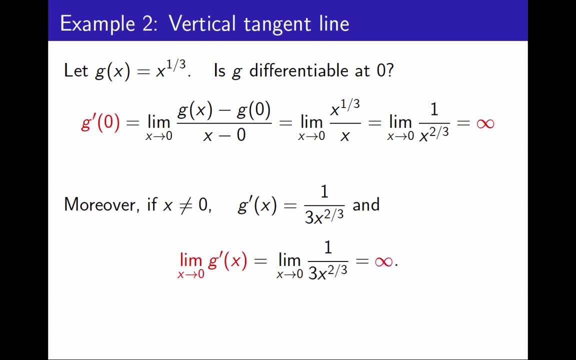 And this limit is also infinity. Perhaps you find that this second calculation is easier than the earlier one. However, a priori, these two quantities, the derivative at 0, and the limit as x approaches 0 of the derivative at x. 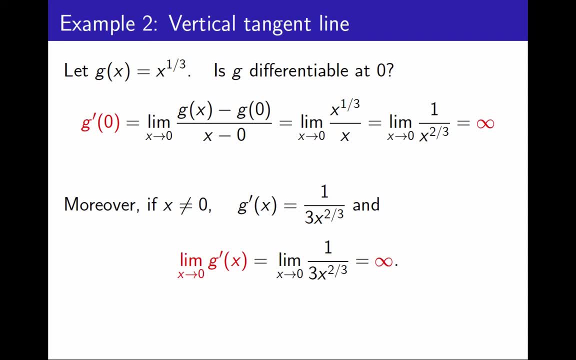 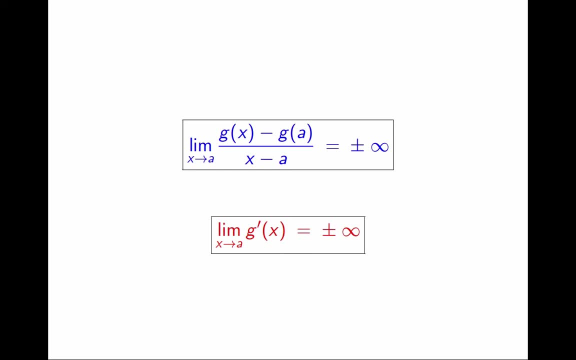 could have been different. They turn out to give the same result. for this example, What is the relation between these two conditions? in general, It is possible to prove that the second condition always implies the first condition. I won't write a proof right now. 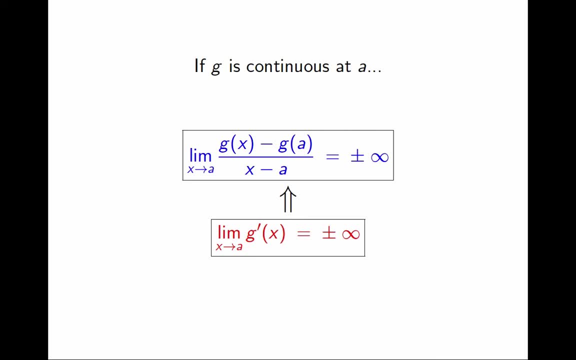 It is an application of L'Hopital's rule To be fair. in practice, for almost all the functions we commonly work with, these two conditions are the same, But if we really insist we can construct some unusual functions that satisfy one but not the other. 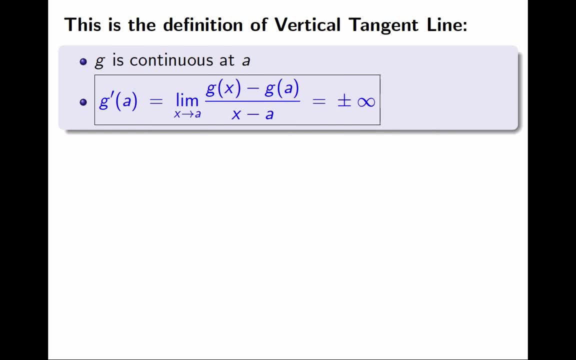 So what do we do with this situation? The correct definition of vertical tangent line requires the derivative to be plus or minus infinity. Requiring instead the limit of the derivative to be plus or minus infinity is slightly stronger, But that is helpful. 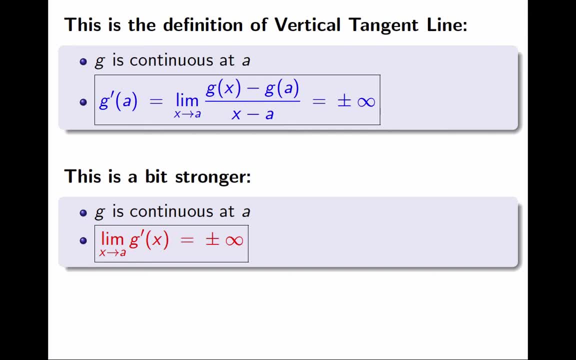 If you are working with an example and you prove it satisfies the second condition, then you have also proven it satisfies the first condition. so you have a vertical tangent line anyway, And that's what we do in calculations most of the time. in practice,